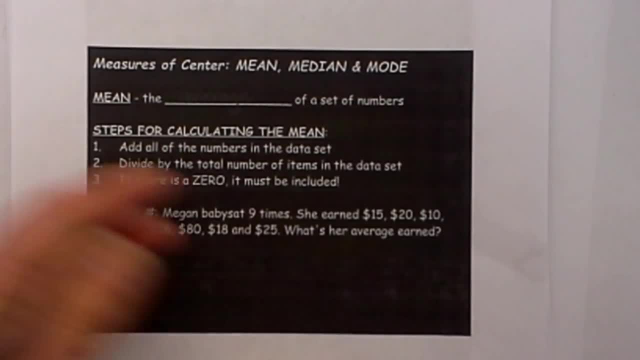 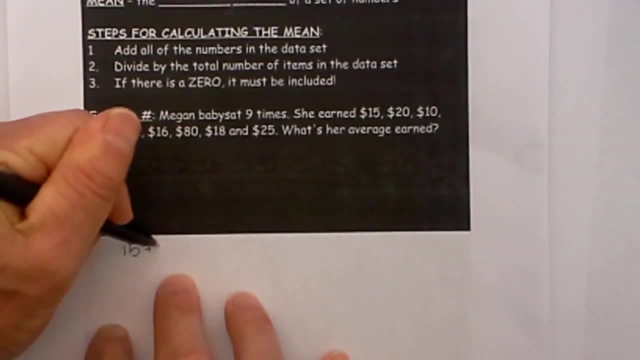 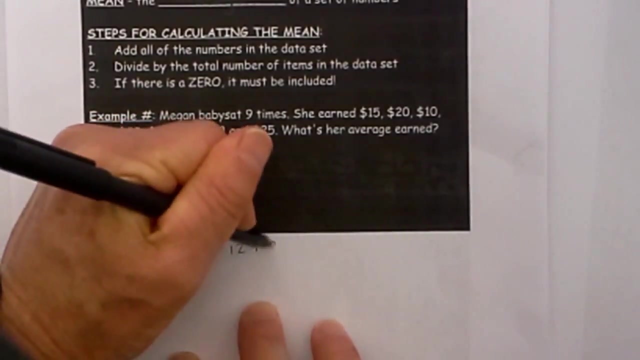 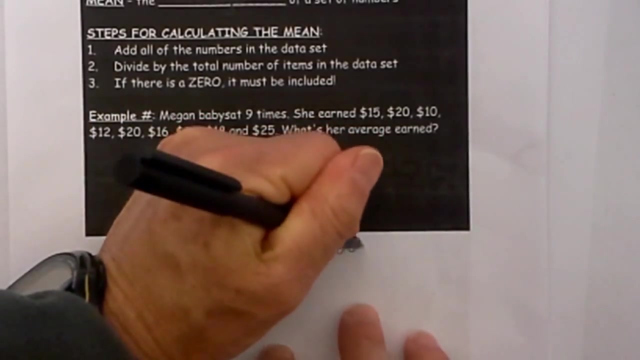 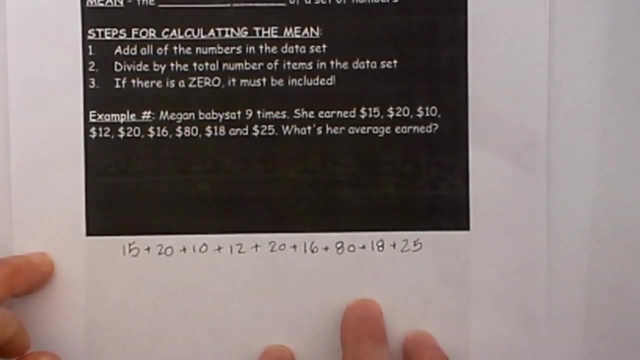 We have Megan babysat 9 times. She earned 15.. She earned 15 plus 20 plus 10 plus 12 plus 20 plus 16.. 16 plus 80 plus 18 plus 25.. If you add all of these numbers together, you get 219. 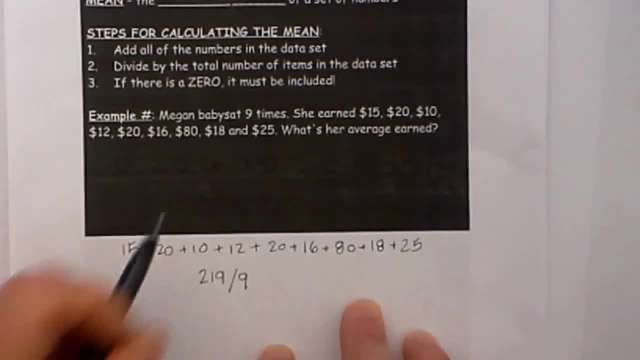 And then we will divide this by 9.. Why 9? Because, remember, divide by the total number of items in the data set And if you count 1,, 2,, 3,, 4,, 5,, 6,, 7,, 8,, 9.. 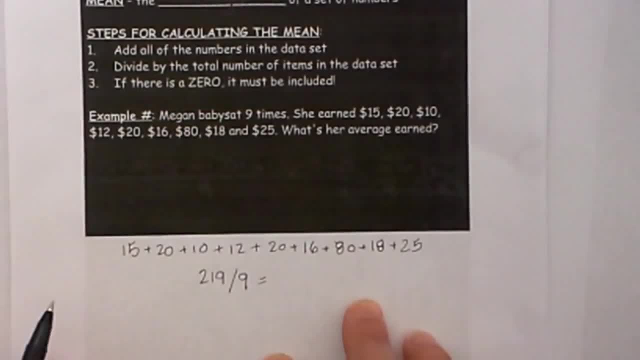 And then you add the total number of items in the data set: 1,, 2,, 3,, 4,, 5,, 6,, 7,, 8,, 9.. And if you divide 219 by 9, that will equal $24.. 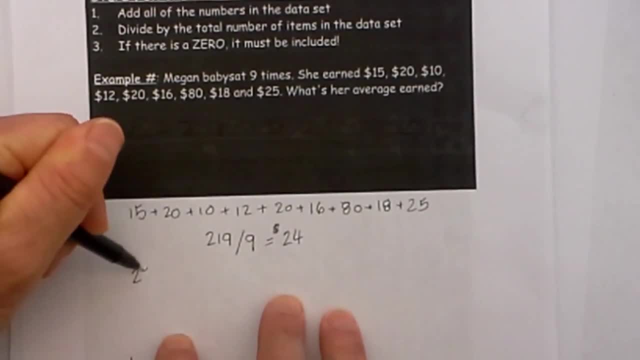 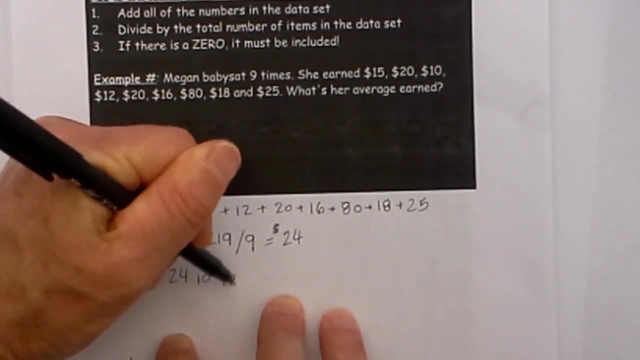 Let's look at another quick example. Say, we have 25 plus 24 and then we have 10,, 12, and 19.. And we want to get the mean of these numbers. Like I started here, you add these together If you add 25 plus 24.. 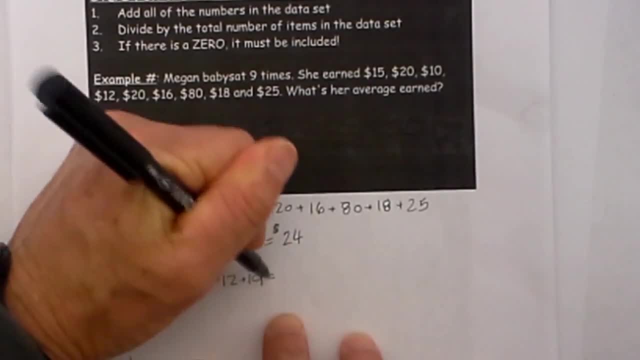 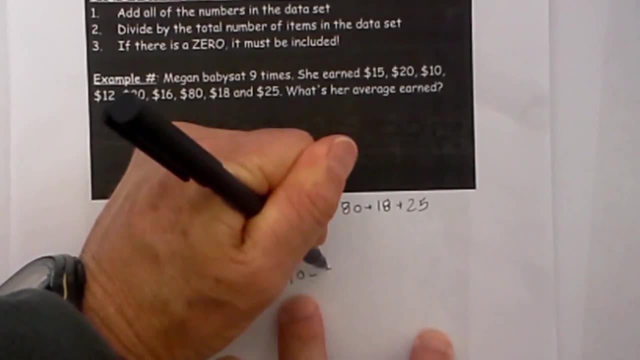 24 plus 10 plus 12 plus 19.. Yes, I did cheat, I added them beforehand. That equals 90 and we are going to divide that by 5.. Again, why 5?? Because 1,, 2,, 3,, 4,, 5.. 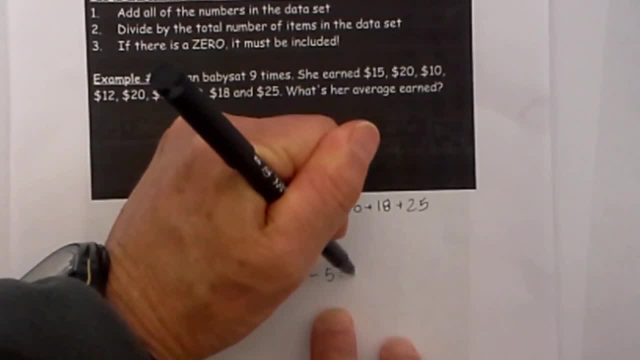 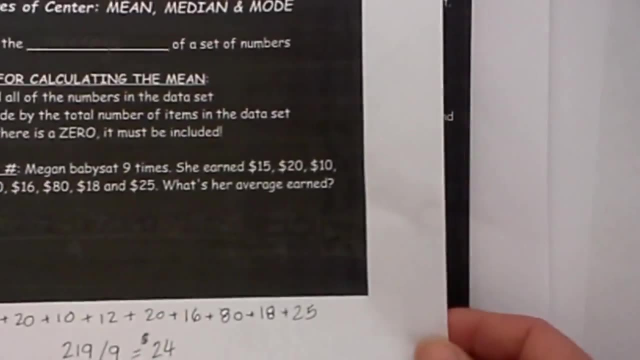 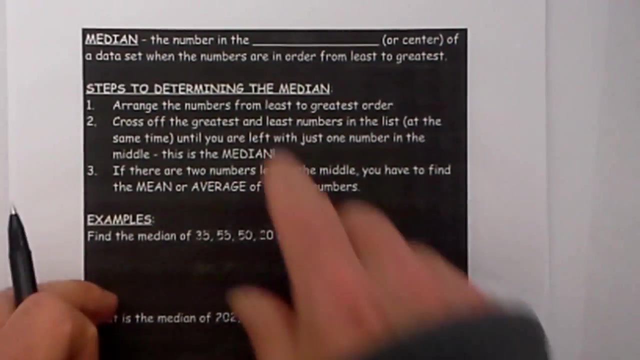 So when I divide 90 by 5, that gives me 18.. And so the mean of these 5 numbers is 18.. Now let's move on to another measure of symmetry Enter, and that is the median. And the median is the number in the middle of a data set. when the numbers are in order, 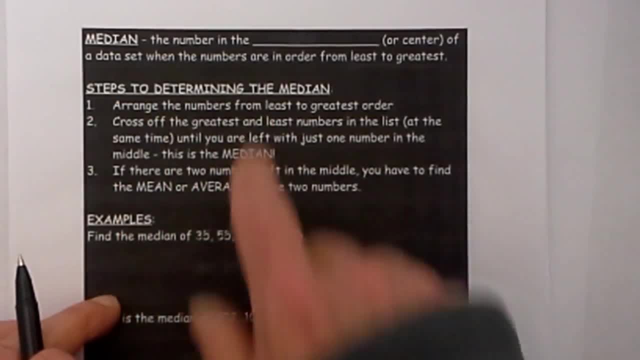 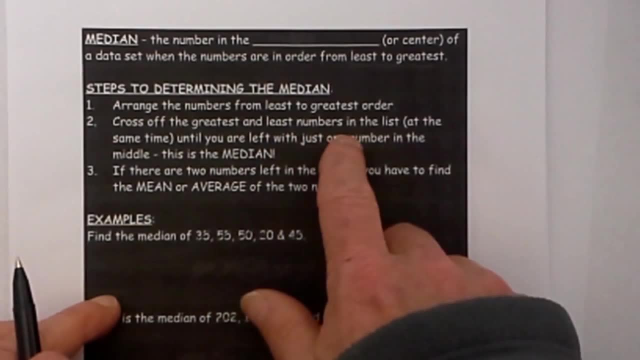 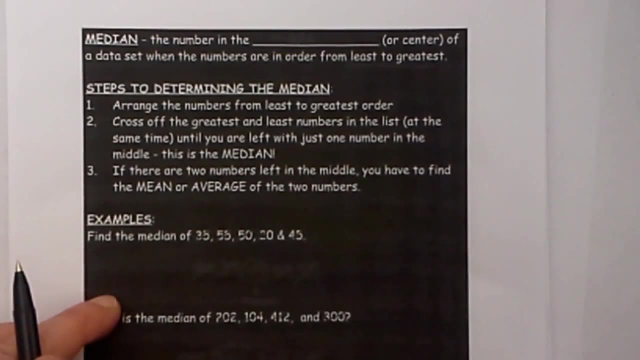 from least to greatest. Steps for determining the median. Arrange the numbers from least to greatest order. Cross off the greatest and least numbers in the list at the same time, until you are left with just one number in the middle. This is the median. 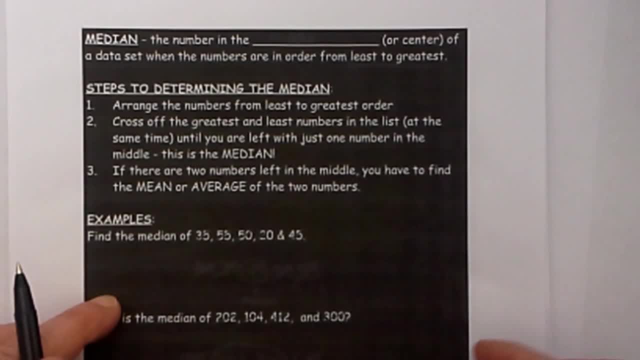 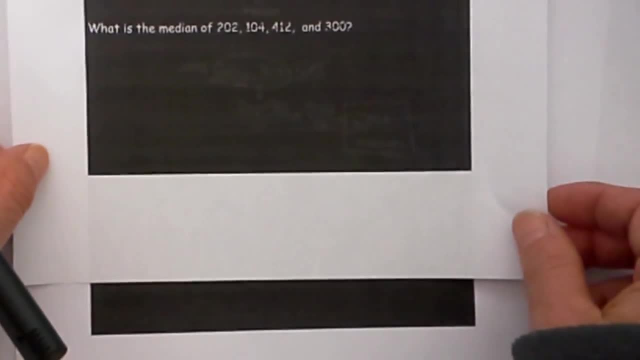 The median. The median, This is the average. The average. There is a two set of numbers. If there are two numbers left in the middle, you have to find the mean or average of the two numbers. So let's go ahead and work 2 sets of numbers. 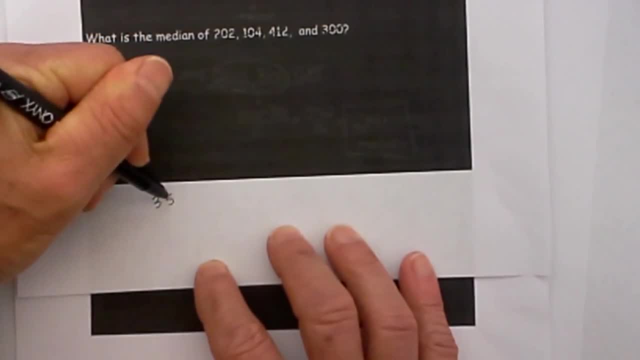 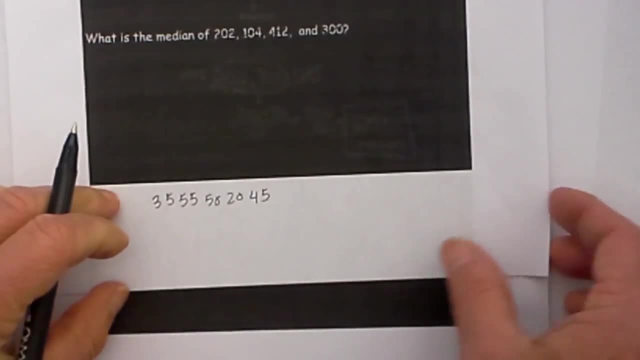 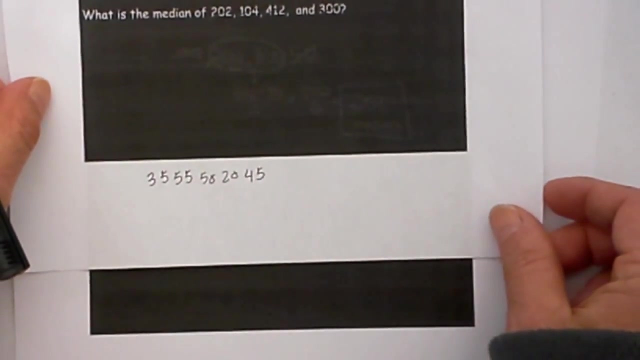 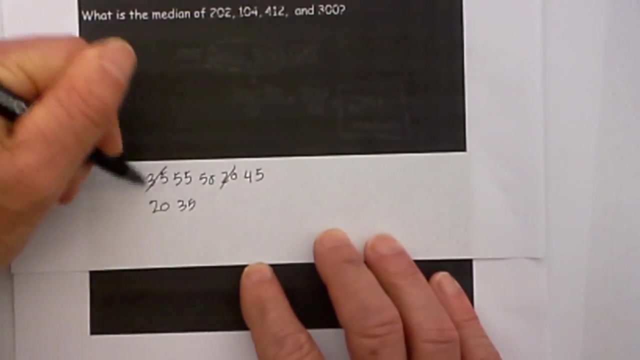 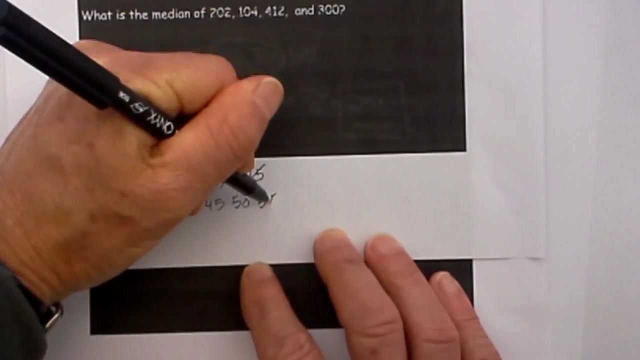 Let's find the median of 35,, 55,, 50,, 20, and 45. And what my steps say is first arrange the numbers from least to greatest. So I will go ahead and do that. So we have 20,, then 35,, then 45,, then 50, and 55. 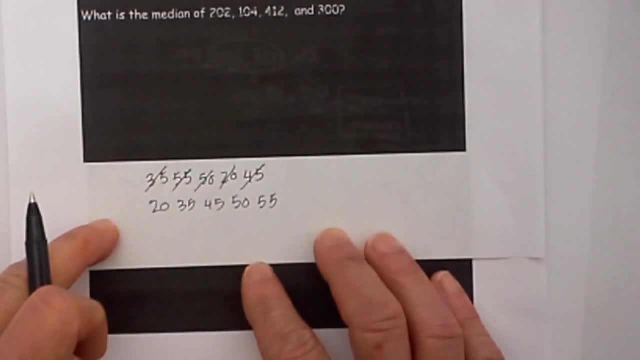 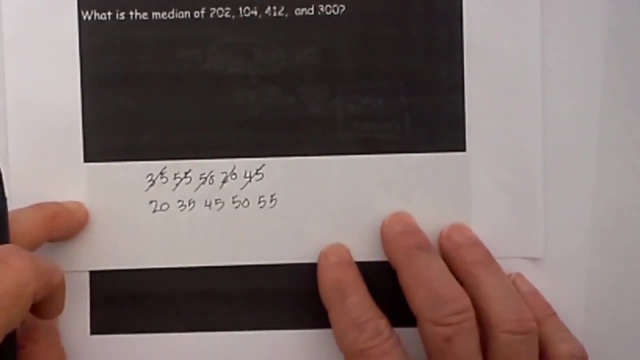 Crossing things off, checking with calculating, especially with several numbers, with median. you need to be careful and not be careless here because you will miss something. So now lets start at the greatest. cross that off and the least, cross that off at the same. 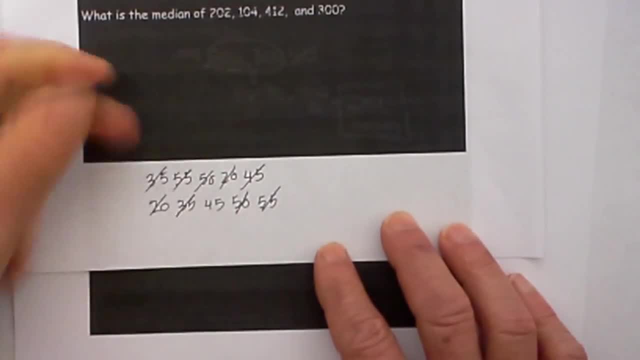 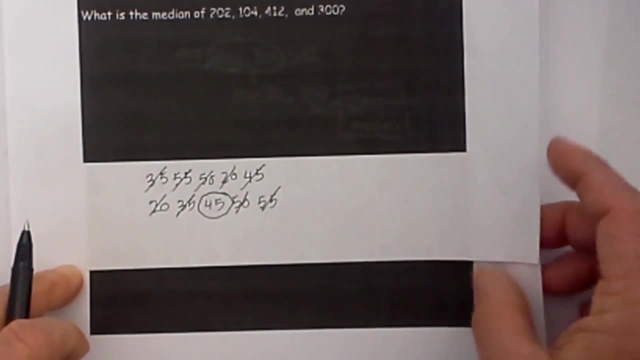 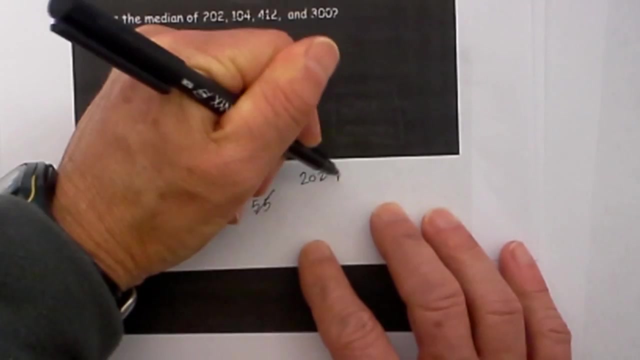 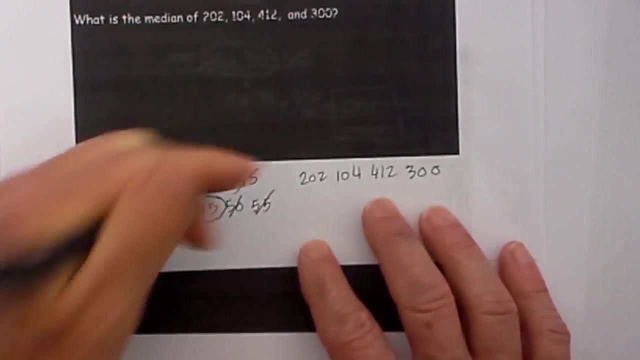 time. Next we will do it again: the greatest and least. and that leaves us with 45, and that is the median. Lets do one more quick example. Lets go with. the numbers are 202,, 104,, 412, and 300. 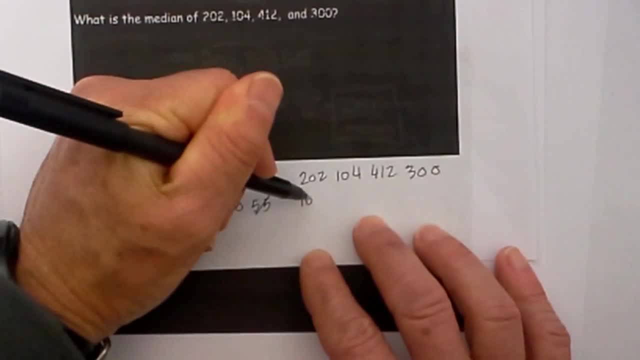 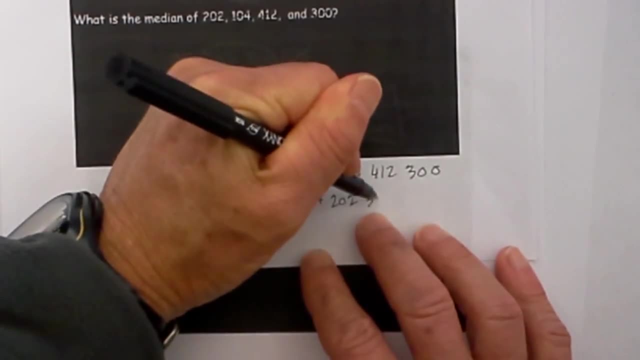 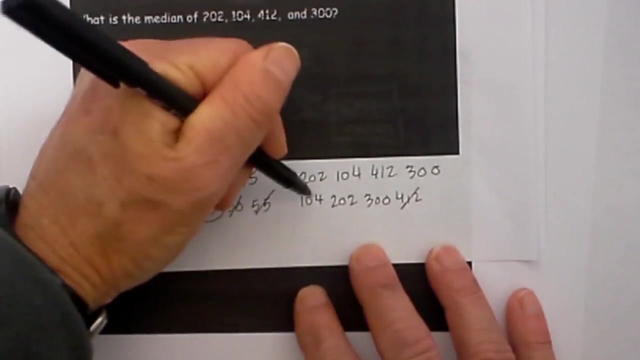 And on this lets first arrange them from least to greatest. So we have 104,, 412, and 300. Then we have 202, and then 300, and 412. And we cross off the greatest and the least and then we are left. we don't have a greatest. 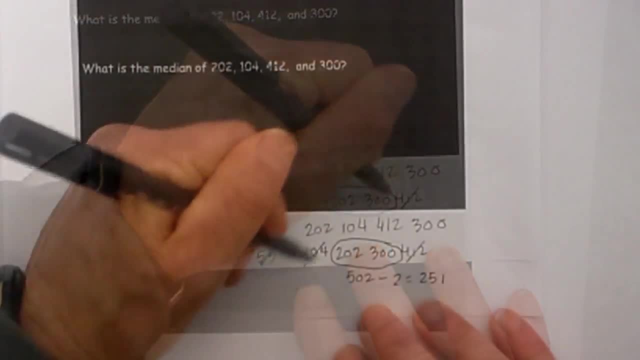 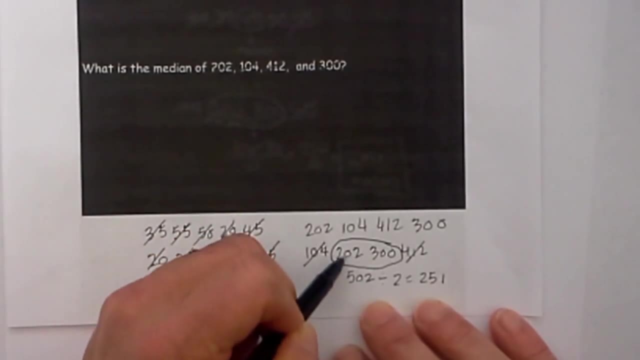 and a least. So we have two numbers. When we cross them off we are left with two numbers in the middle. So now we need to take the mean of these two numbers. So when I add 202 and 300, that is 519.. 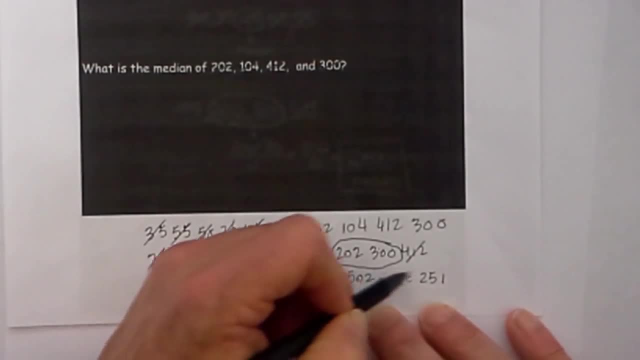 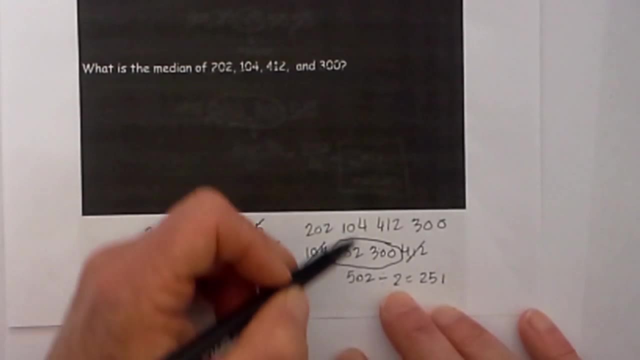 And then I add 202 and 300. That is 519.. That is 251.. Why did I use 251? Because, remember, when you are calculating the mean, you total the numbers and divide by the number of numbers in the data set, and that is 2.. 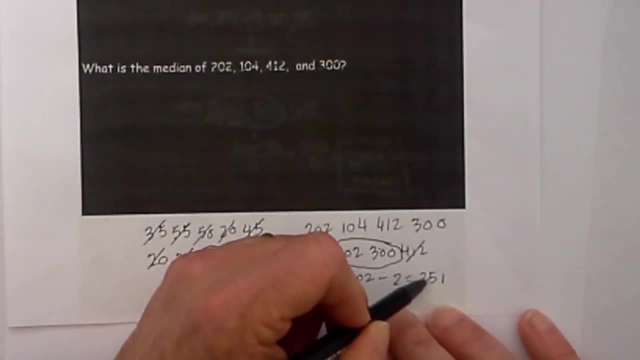 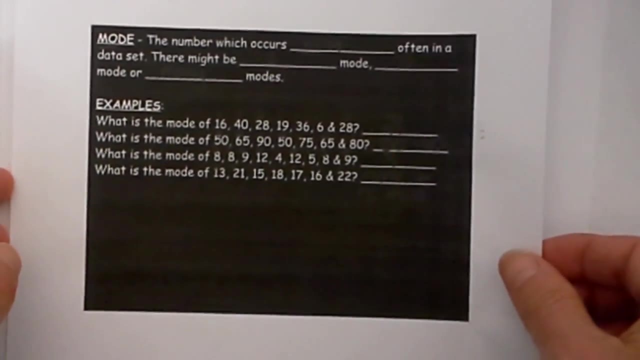 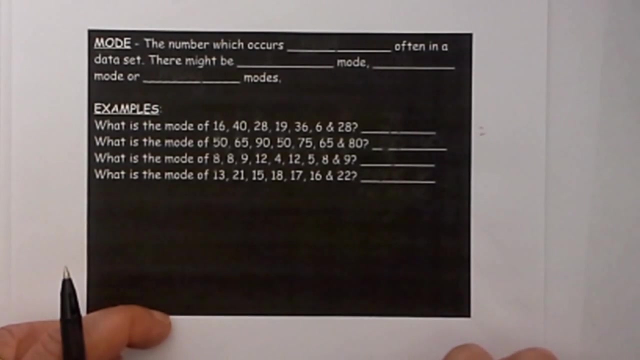 So, anyway, the median of these groups of numbers would be 251.. So now lets move to the last section, and that is calculating the mode. And the mode is the number of numbers, The number which occurs most often in a data set. There might be one mode, more than one mode or no mode. 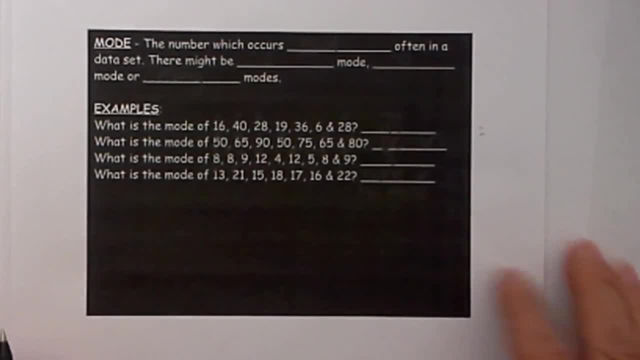 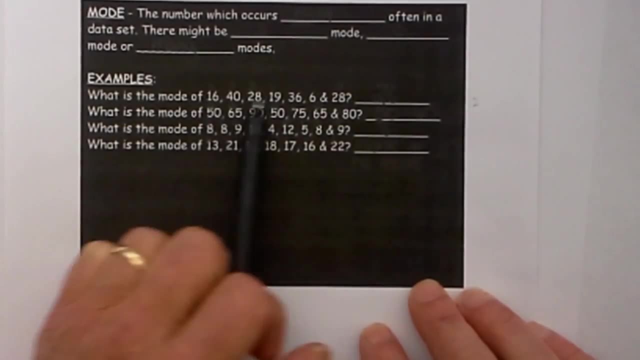 So lets look at an example, and I have an example in each one of these And I am going to go ahead. lets just go through. If we look at this 16, if you look carefully, it only occurs once 40 occurs once 28 occurs. 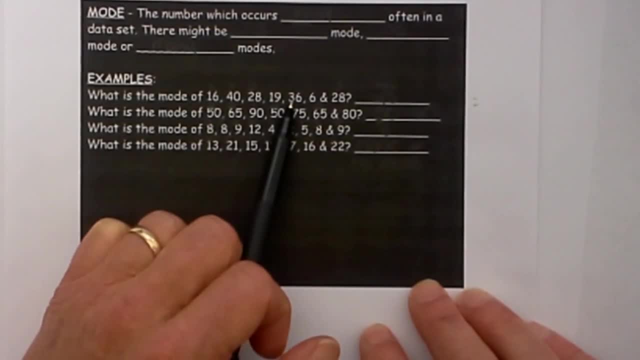 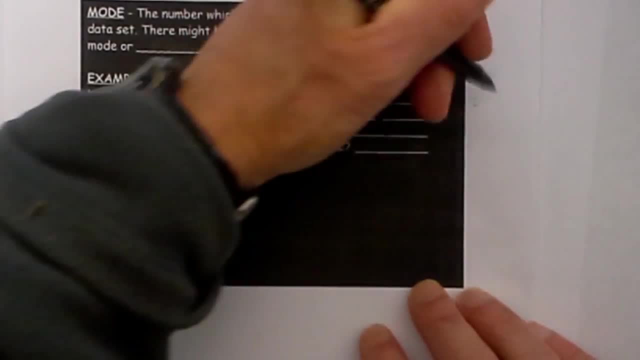 once, 2.. 19 occurs once, 36 occurs once and 6 does So the mode of this set of numbers- 16,, 40,, 28,, 19, etc. is 28.. Lets move down to the next set quickly. 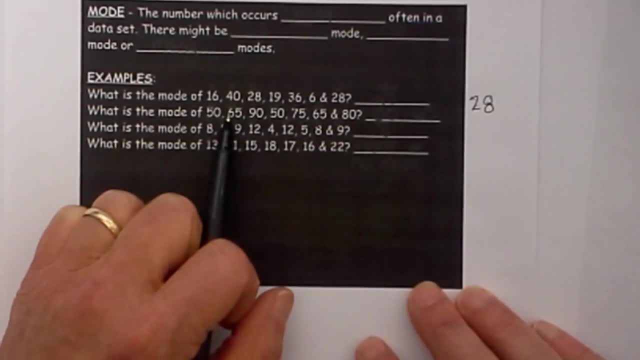 We have 50, it is 1 two times 65 is 1 two times 90 is once, 75 is once 80. So in this one we have more than one, We have 50. And 1.. 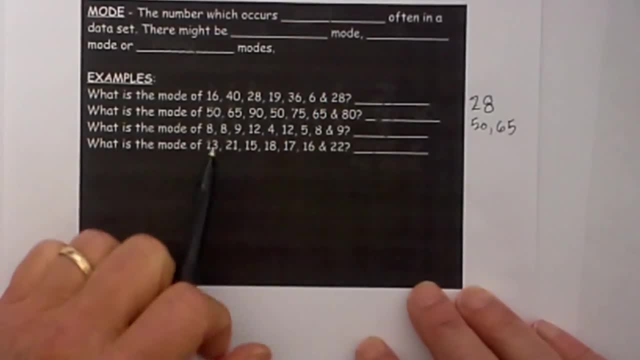 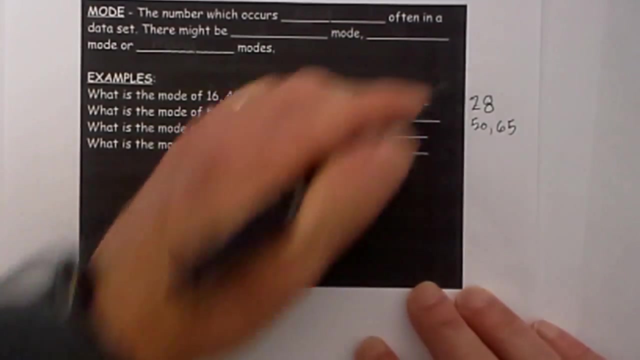 65.. This next one: we have 8, 1,, 2, 3 times, 9, 2 times 12, 2 times and 4 one time. So since 8 occurred 3 times in this example, it will be 8.. 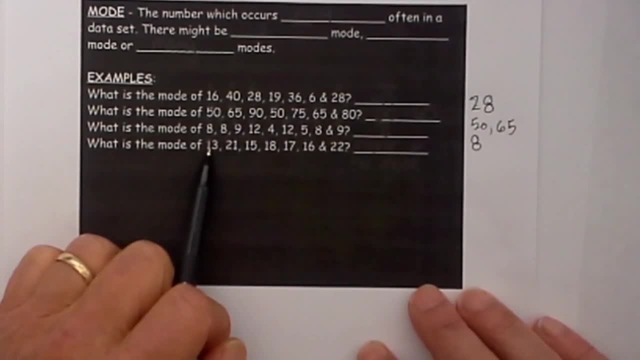 And last but not least, lets look at this next example. We have 13 occurs once 21, once 15, once 18, once 17, once 16, once 22.. So there is none, There is not a number. that occurs most often. 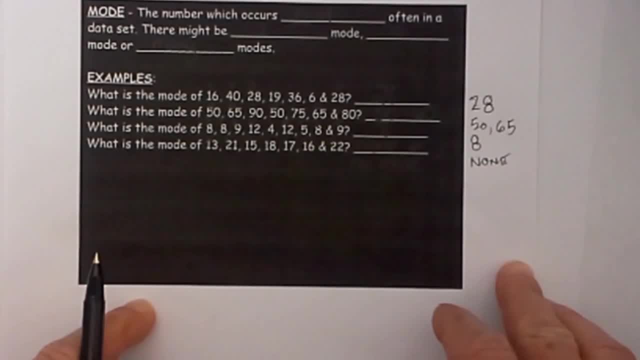 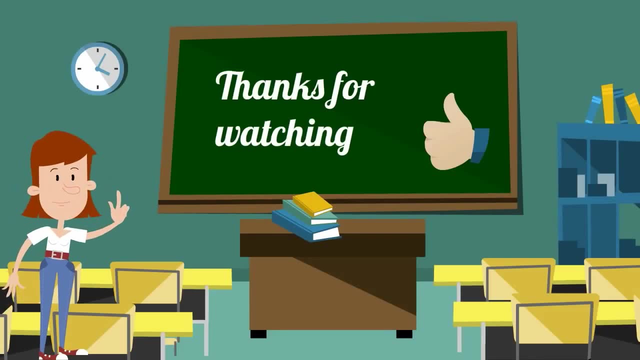 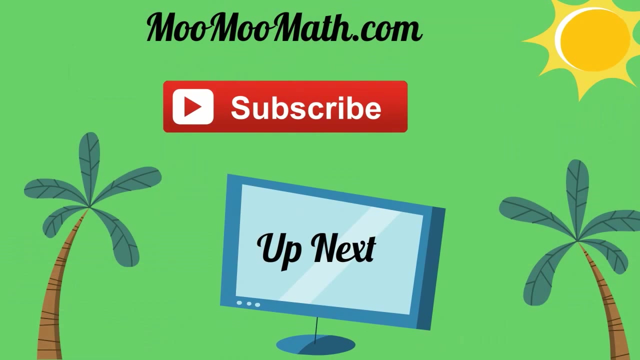 They occur. the same Hope that helps with measure of center. MooMooMath uploads a new Math video every day. Please subscribe and share, Thank you. Thank you for watching. See you next time.